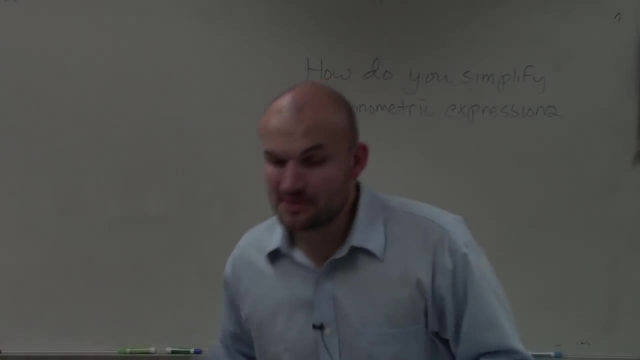 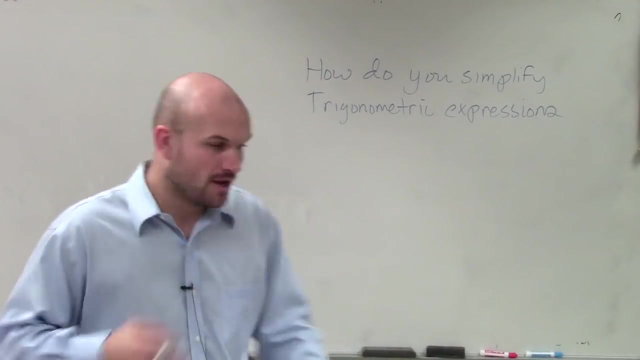 Welcome. So how do we simplify trigonometric expressions and what is really going to be kind of the process that we're going to want to follow? Well, you know, very similar to what we learned when we first started doing like order of operations to simplify numeric. 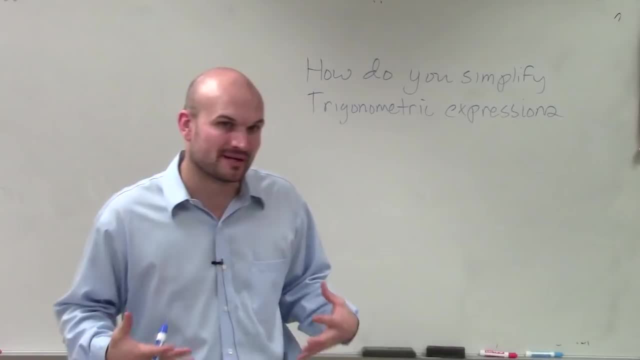 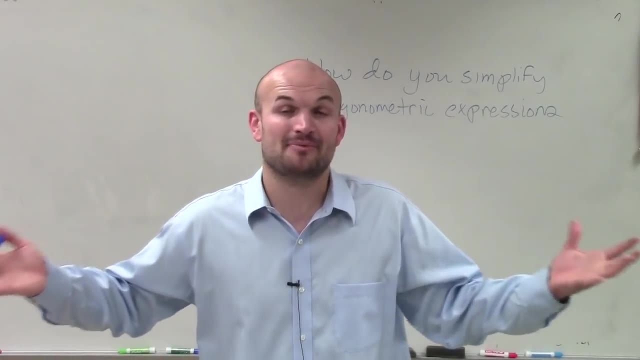 and algebraic expressions. we're going to be using a lot of those properties to go through this And to simplify trigonometric expressions. what we're going to want to do is take our complicated expression and simplify it to its simplest form, usually trying to written. 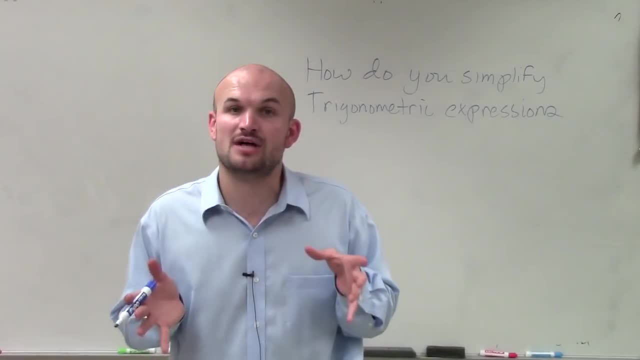 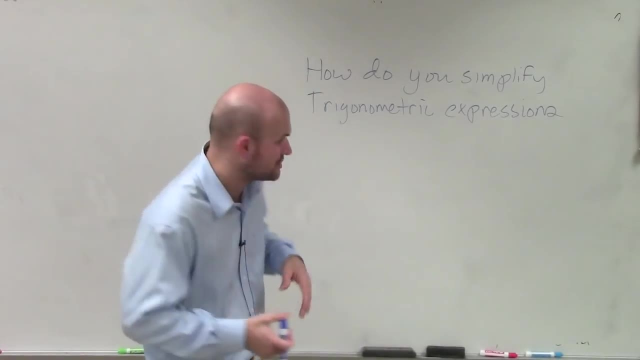 out in either as a form, as a number, or in its simplest function, of either one or two functions either combined or as least as one expression. So to do that, there's a lot of things that you're going to have to start looking into, And I want to kind of go through. 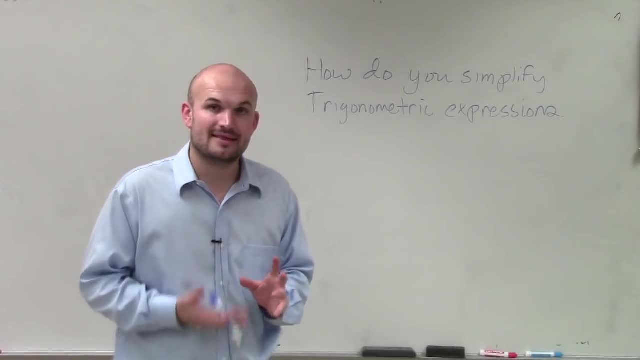 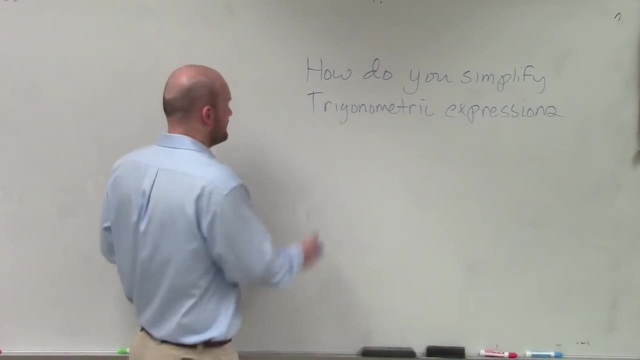 a couple main points that I see in algebra that I want to make sure students remember as far as how to do it, How we're going to apply them in our trigonometric expressions. The first one is our reciprocal property. You know, if we have x over y times 1 over x, remember we can rewrite that as: 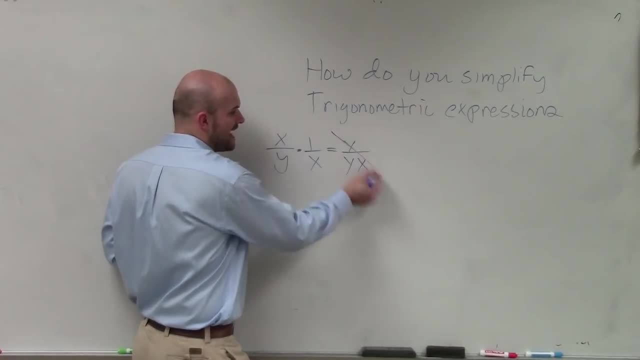 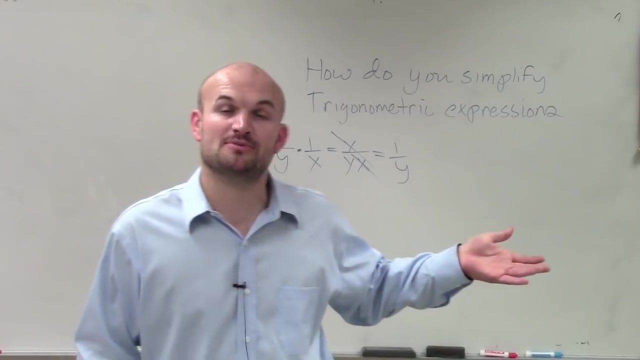 x divided by y over x. Therefore, the x's are now going to divide to 1 and I'm just left with 1 over y. So it's very important, especially when we're looking into multiplying rational expressions or we just have one rational expression. we always want to look for that. 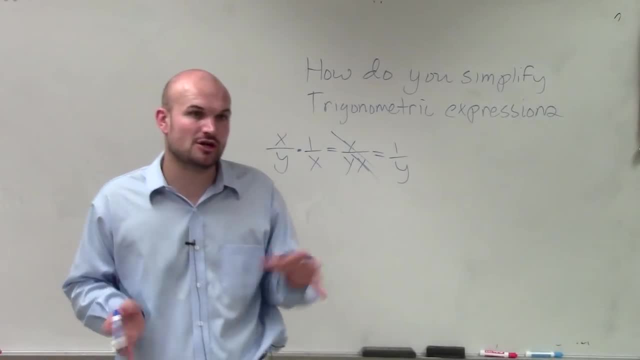 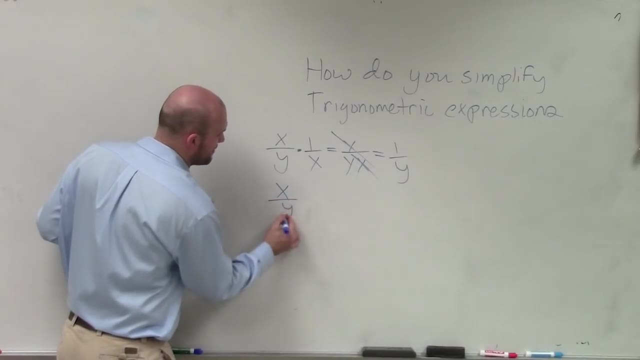 opportunity to be able to divide out our trigonometric terms so they can equal 1.. This also comes up when we have maybe complex. So let's say, if I had x divided by y divided by z, All right. So a lot of times what we want to do for this one is again look for our reciprocals. 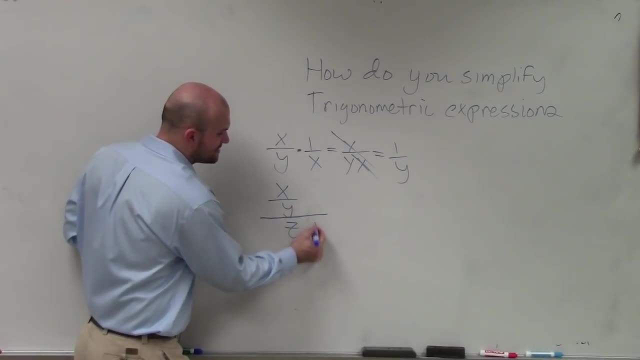 So if I have x divided by y divided by z, I can multiply this by 1 over z, Again by multiplying this by my reciprocal that divides to 1.. And then I'm left with multiplying by the reciprocal and the denominator and the numerator, where my final answer would be: 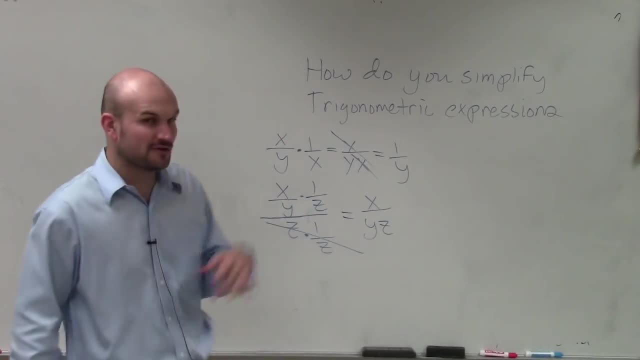 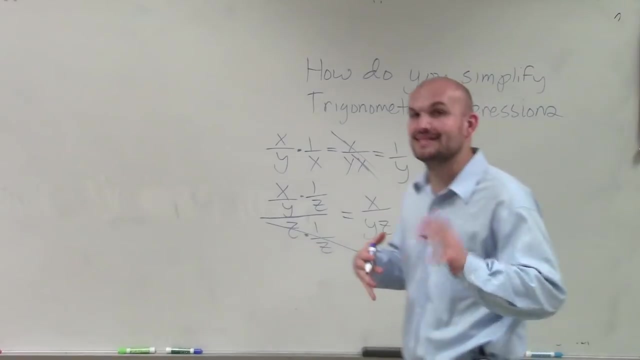 x over y times z, All right. So those are some very important skills when dealing with fractions and your reciprocals. But that's not the only take that we're going to be using for simplifying our trigonometric identities. One thing we're also going to go through is 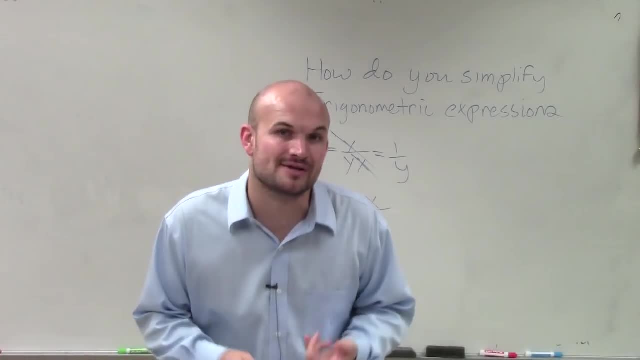 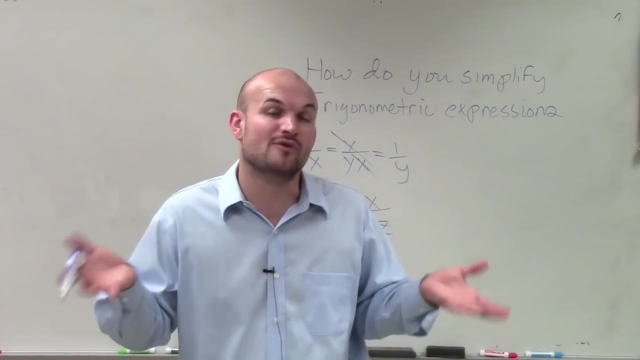 factoring. You need to remember how to make sure you can factor the difference of two squares, Make sure you can factor by using our AC method or just be able to factor a regular trinomial When our coefficient of a equals 1,. they're going to come up. We're going to want to go. 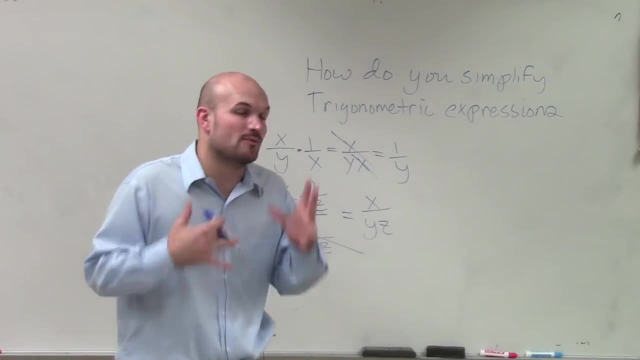 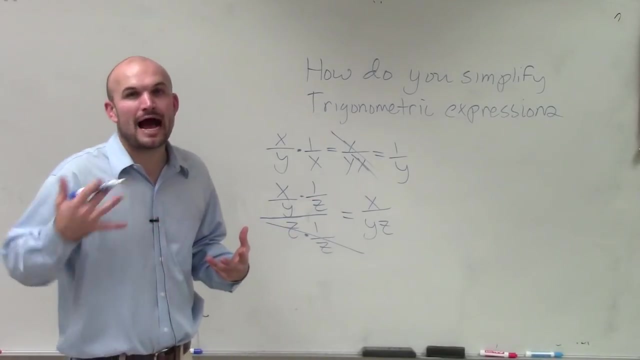 ahead and use them, And what we do is when we simplify or when we use our factoring. the main important thing about simplifying trigonometric expressions is looking for the opportunity to use our identities, And again the identities which have previously been. 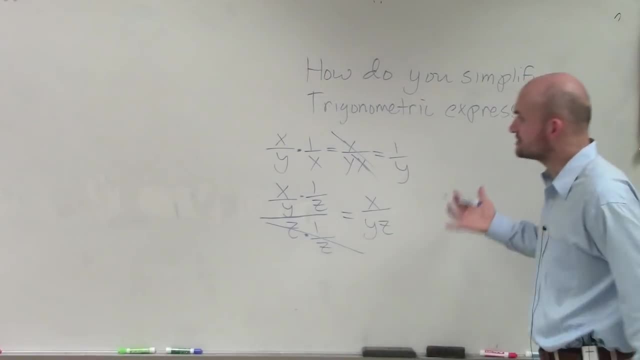 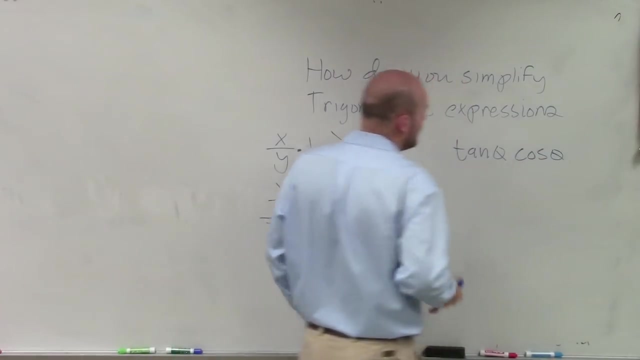 given to you guys have a reference sheet. You're going to want to use those identities to substitute them into an equation, So therefore you now produce maybe a fraction. So, for instance, if I had like tangent of theta times cosine of theta. Well, if I wanted to simplify this, 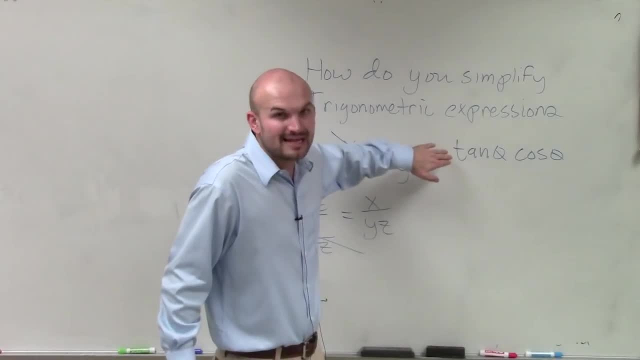 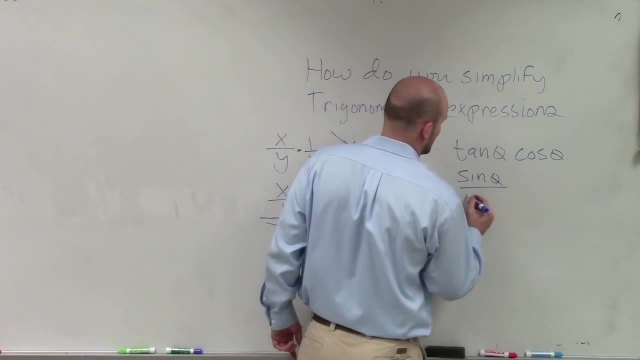 I can use my quotient identity to say: all right, well, let's rewrite this, Let's get this into some fractions. so maybe then I can simplify this out, So I can rewrite the tangent as sine of theta over cosine of theta, times cosine of theta. 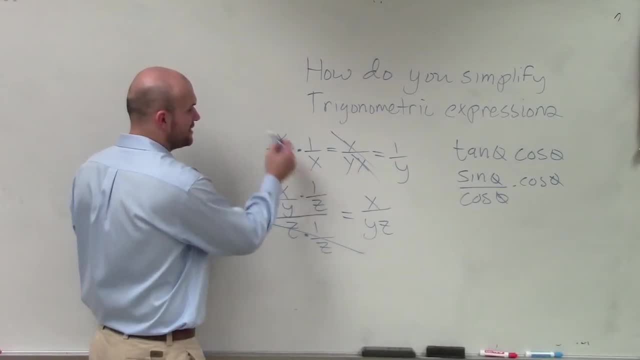 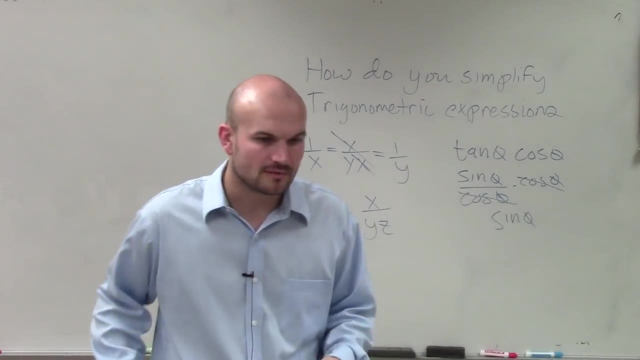 Now I have a similar operation, like I had over here, where now the cosines are going divide out and I'm just left with one trigonometric term of sine. So that's going to be very important when you're looking for these You're always going to want to be using. 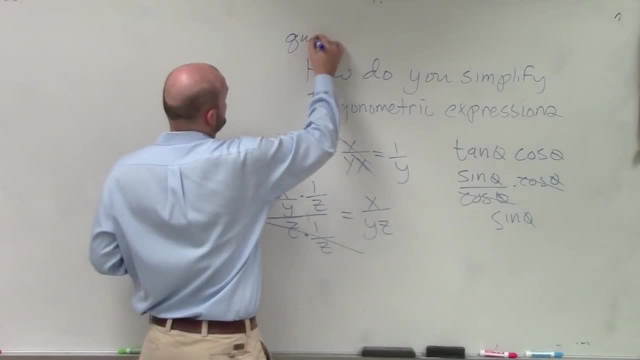 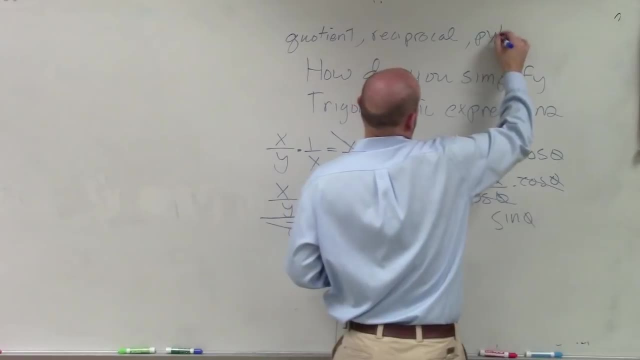 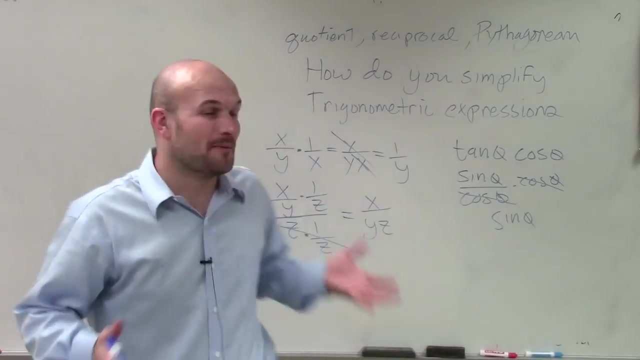 think about the main ones that I would like to say is your quotient reciprocal or Pythagorean, Because I can give him the big P, because he's a big guy. Those are going to be your main identities that you're going to be using. 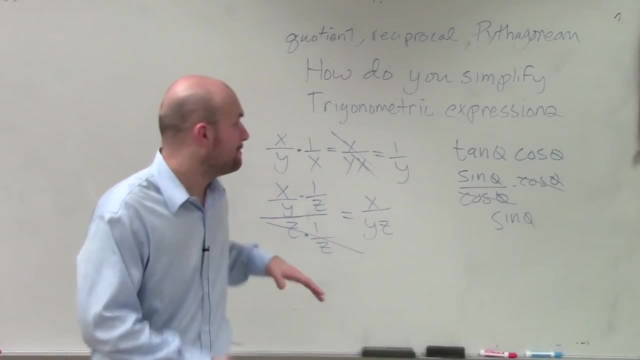 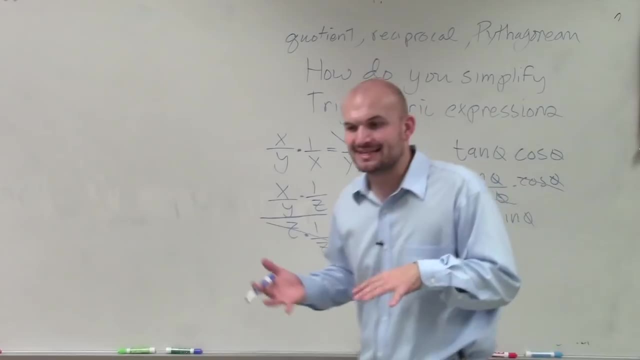 You're going to use co-function, You're going to use even and odd, But those are going to be your main functions, that, almost on every single problem, you're going to want to apply And you're going to want to substitute. And the great thing about simplifying expressions. 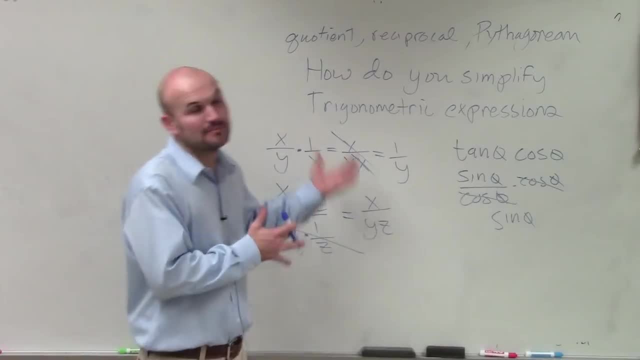 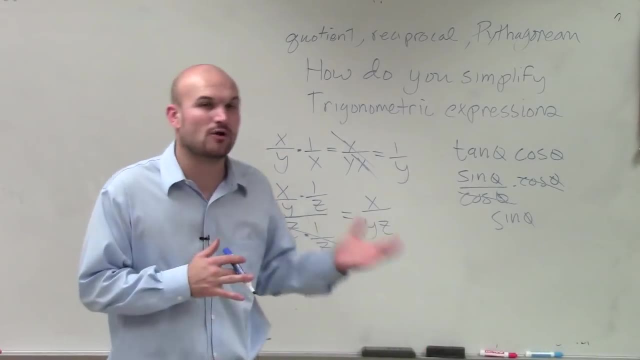 is. it's all about just trying, See how far you can get. Try something, And if it doesn't work out, try maybe substituting in a different identity and see where it's at. There's not always great right or wrong answers. 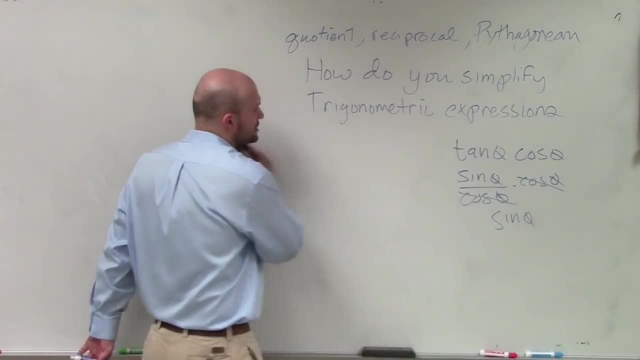 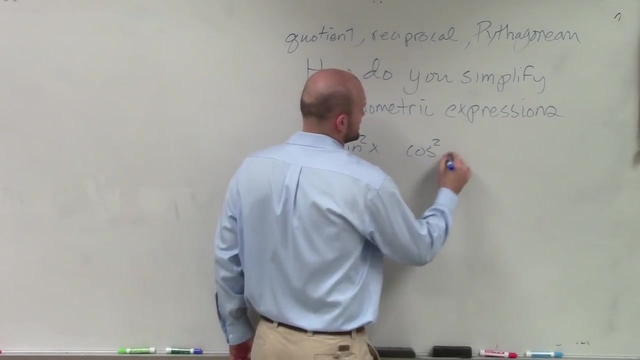 But one thing I do want to talk about, for you to look for when you're doing, when you're simplifying your chicken metric identities, is looking for these terms of sine squared of x, cosine squared of x or tangent squared of x. 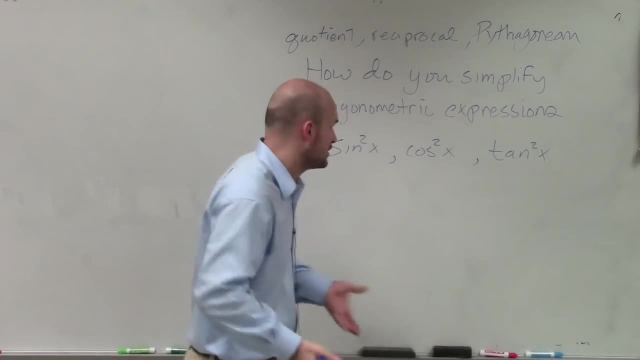 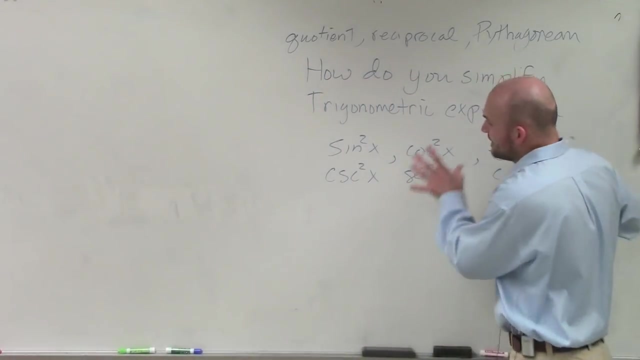 When you see any one of these trigonometric terms, what I always think, or actually even their reciprocal identities. there's not a lot that we use with these true identities in simplifying trigonometric expressions. So whenever I see any of these terms squared, 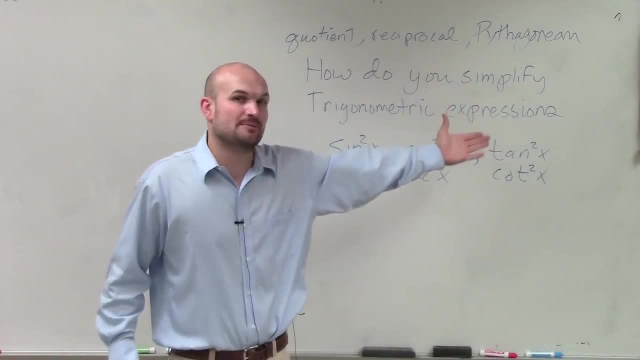 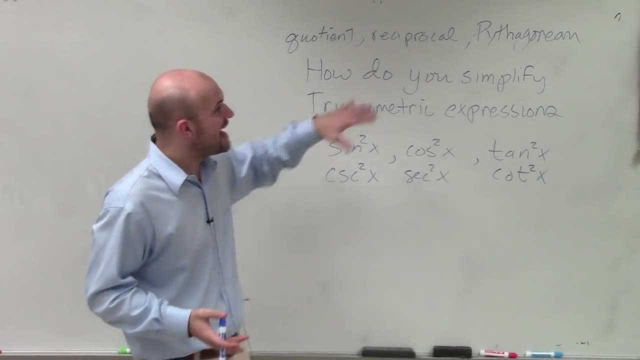 I automatically, I automatically think I'm going to try to replace it with the Pythagorean identity. Now, not always is that the best solution or the best thing to do, but a lot of the times that is going to get something moving where. 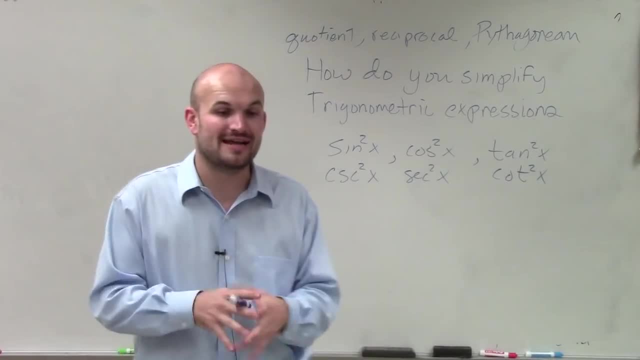 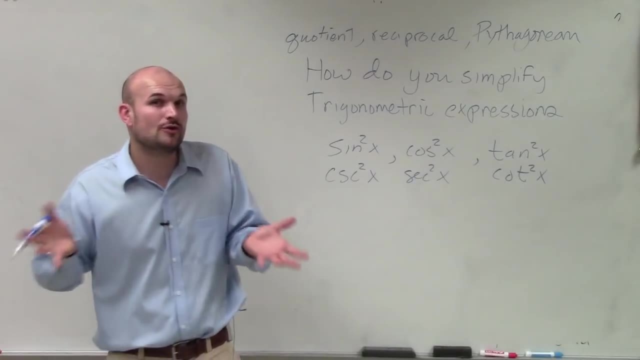 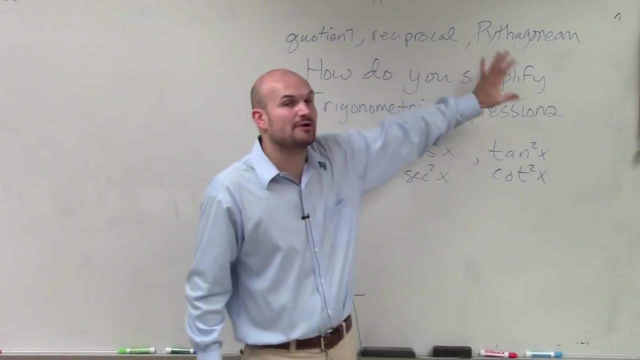 you're going to be able to finally simplify your expression. You're finally going to get maybe the same terms on the numerator and denominator that you can divide out. So look for those opportunities for when you have these functions that are squared, Look to try to apply. 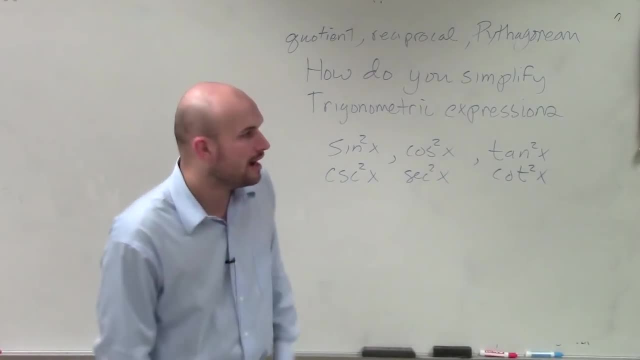 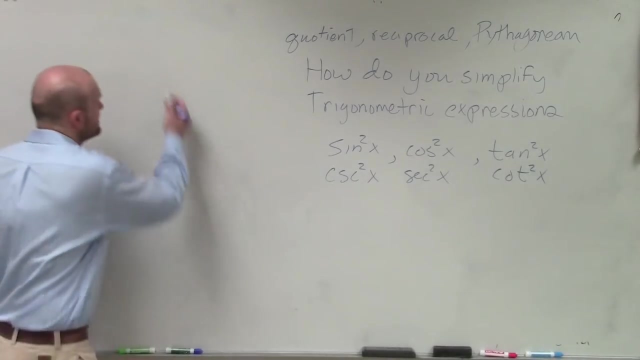 You're Pythagorean identities to substitute in those values. Also, try looking for opportunities to create a sine squared, cosine squared and so forth. For instance, if I have 1 over cosine of theta minus 1, well, if I go ahead and simplify this, I don't know. 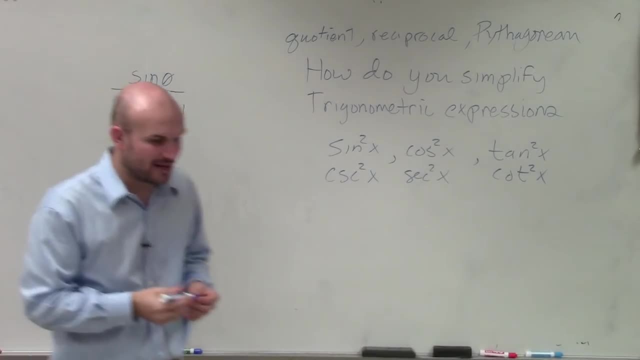 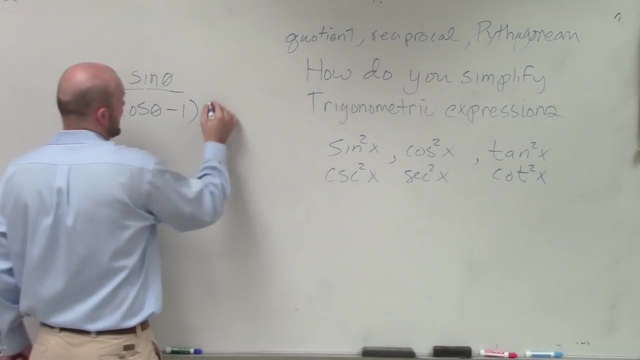 let's do sine or something. I'm just totally making something up, But right now there's really nothing I can do to simplify that. However, if I go ahead and multiply my denominator by cosine of theta plus 1, now what I've created in my denominator. 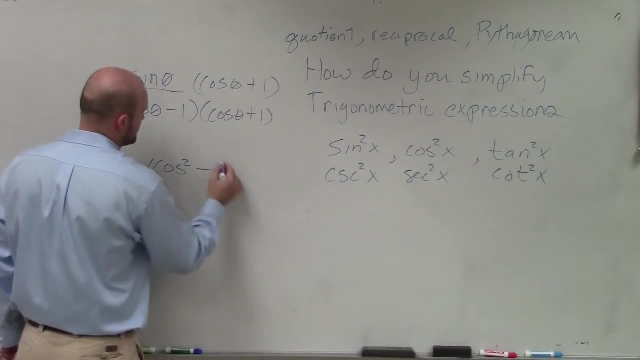 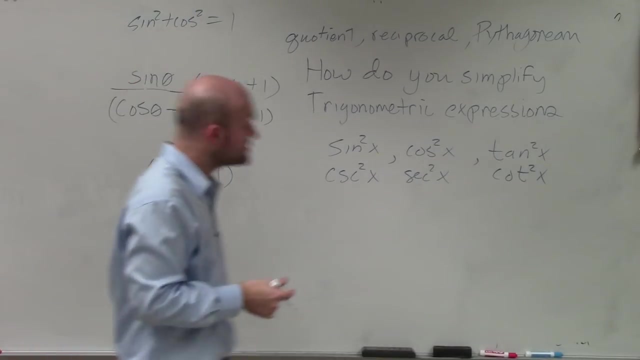 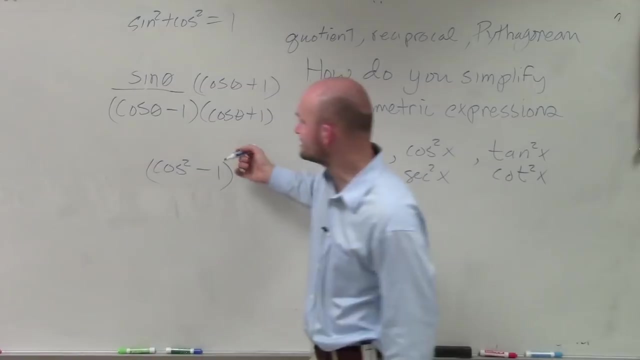 is cosine squared minus 1.. And we know that sine squared plus cosine squared equals 1.. That is your trigonometric expression. So now, by go ahead and rewriting this, I could now replace this in my denominator, because I have 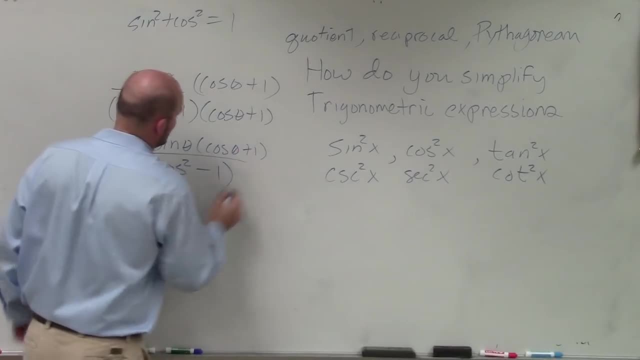 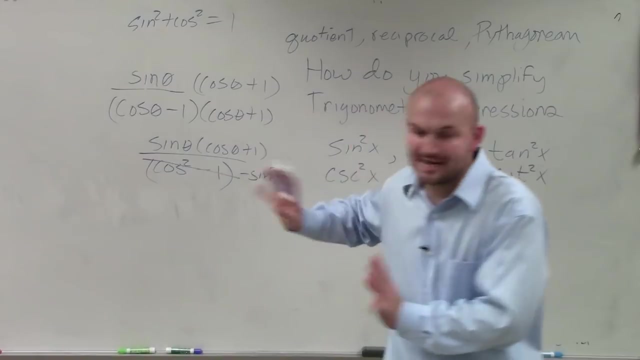 sine of theta times cosine of theta plus 1.. I can now rewrite cosine of negative 1 as negative sine squared of theta. Now how that's going to affect the rest of that problem. I just kind of made that up, for instance. 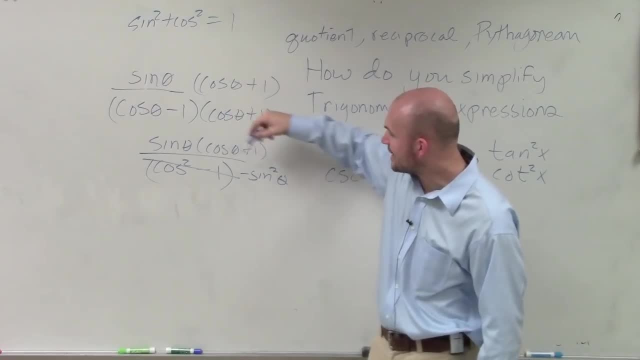 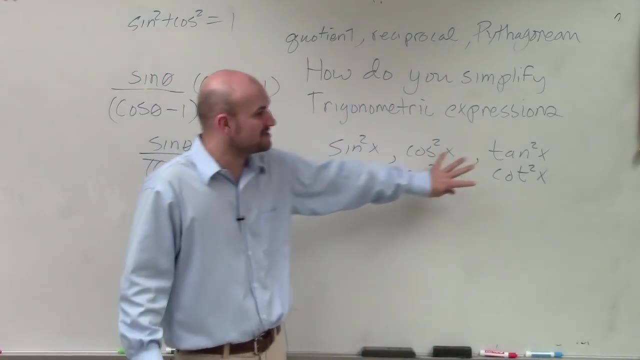 But then you'd be able to delete out a sine, Then you'd have a cosine over sine which you convert to a tangent, And then you might possibly have a trigonometric identity, which is a tangent, And then you'd have a tangent or a cotangent. 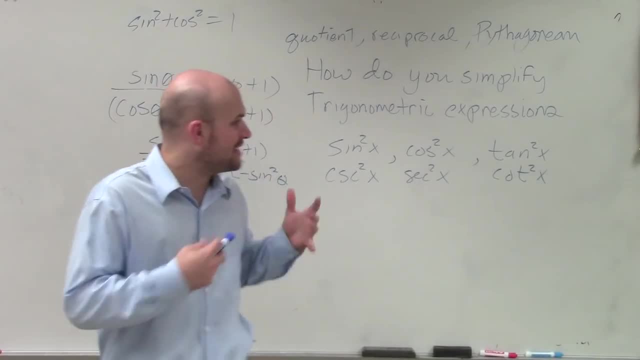 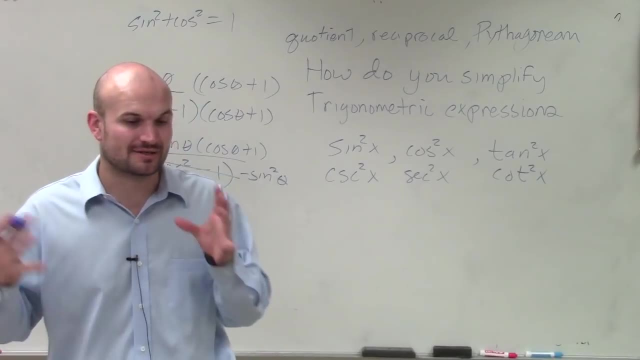 So you've just got to start looking at the box And I would just say in general, when looking through these problems, it's just going to start trying things. Try it, See how far you can get. Make sure you're applying your identities.